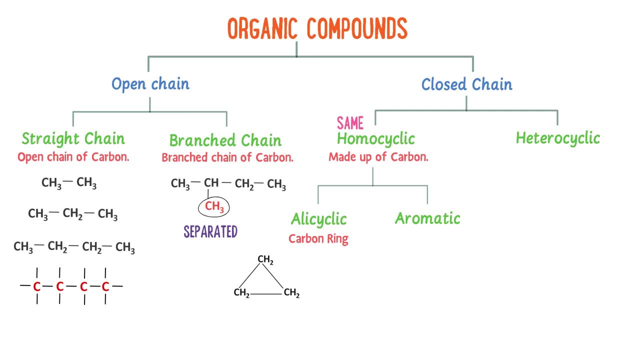 a ring, for example, cyclopropane, cyclobutane, etc. The structure of cyclopropane is like a triangle. The structure of cyclobutane is like a square. We can see that the structure of all these organic compounds are cyclic, which contain: 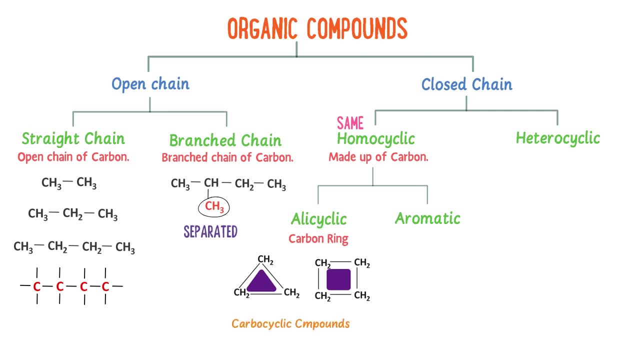 carbon ring. That's why we call them carbocyclic compounds. That's why we call them carbocyclic compounds. That's why we call them carbocyclic compounds. Secondly, aromatic compounds are those organic compounds which contain alternate single and double bond between the carbon atoms, for example benzene. 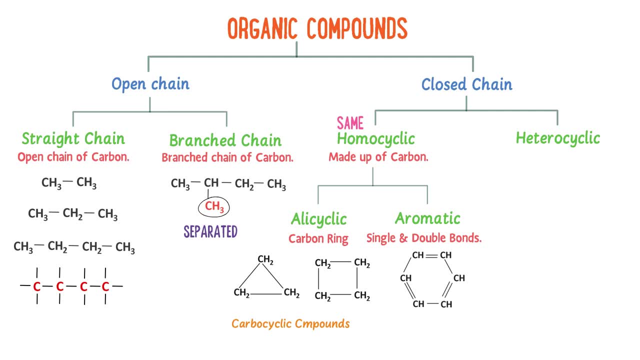 In this organic compound, carbon atoms are joined together by alternate single and double bond. It also contain only carbon ring, so it is also known as a carbocyclic organic compound. Thus, remember that homocyclic organic compounds are divided into heterocyclic and heterocyclic. 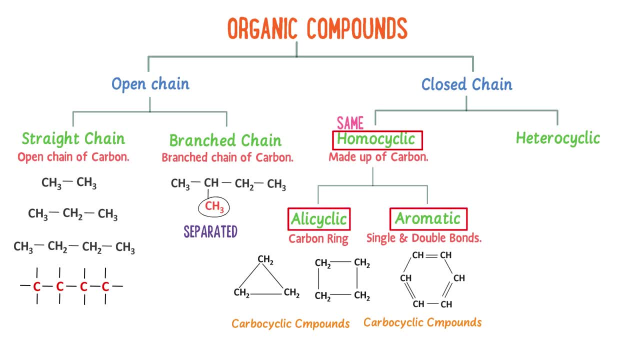 organic compounds. The heterocyclic organic compounds contain carbon ring, having single bonds, while aromatic organic compounds also contain carbon ring, but having alternate single and double bonds. Now, what about heterocyclic organic compounds? Well, the word hetero means different. So hetero cyclic are those organic compounds whose ring is made up of one or more atoms. 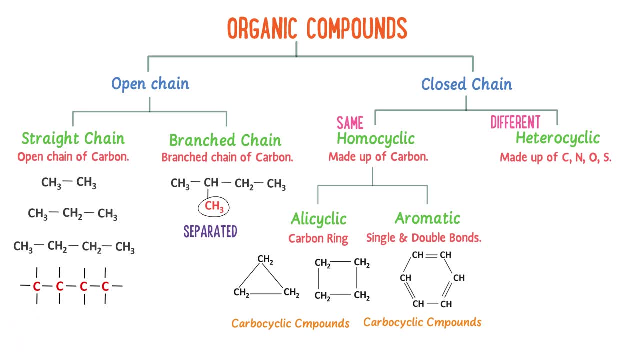 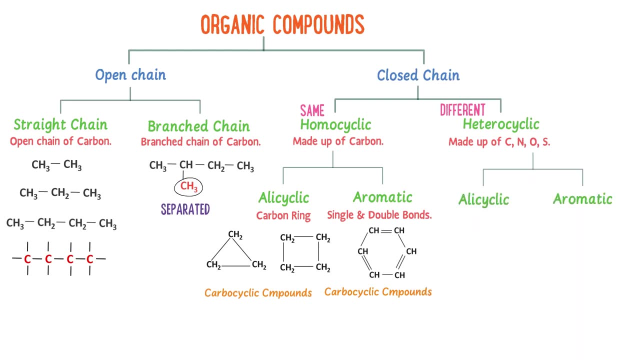 like nitrogen, oxygen, sulfur, etc. Heterocyclic organic compounds are further divided into helicyclic and aromatic organic compounds. Helicyclic are those organic compounds which contain one or more atoms in their ring, like nitrogen, oxygen and sulfur, but they have single bond. 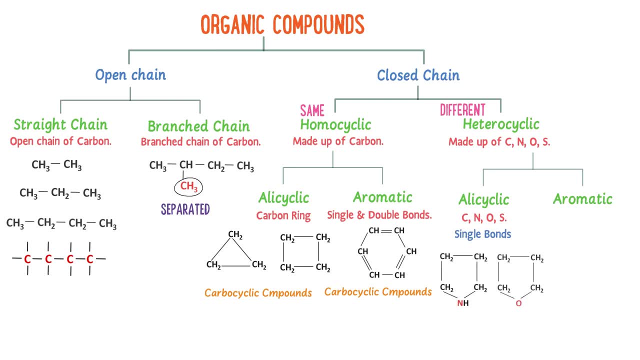 For example tetrahydropyrrole and tetrahydrofuran. We can see that these rings contain either sulfur, nitrogen or oxygen atom in their respective rings, but they all have single bonds. Therefore, we call these organic compounds as heterocyclic organic compounds. 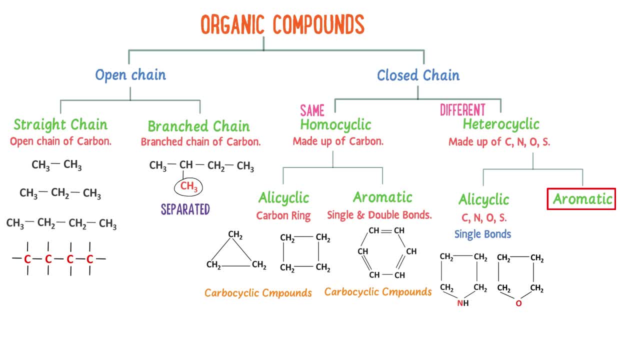 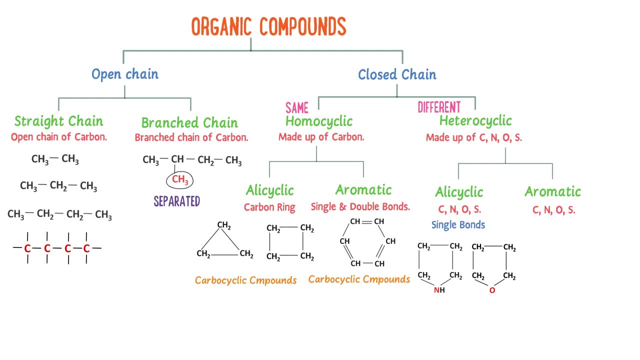 Secondly, aromatic organic compounds are those compounds which contain one or more atoms like nitrogen, oxygen, sulfur, in their rings, but they have alternate bonds, For example, tetrahydrofuran and tetrahydrofuran. For example, tetrahydrofuran and tetrahydrofuran.